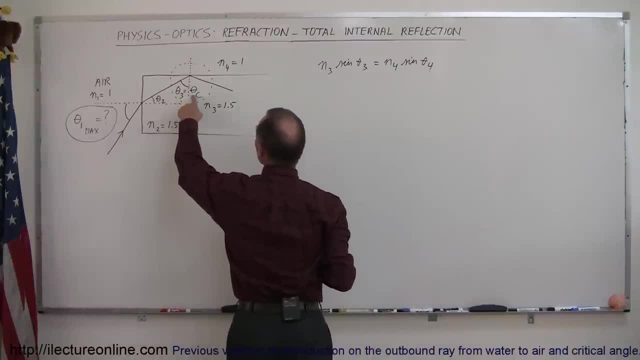 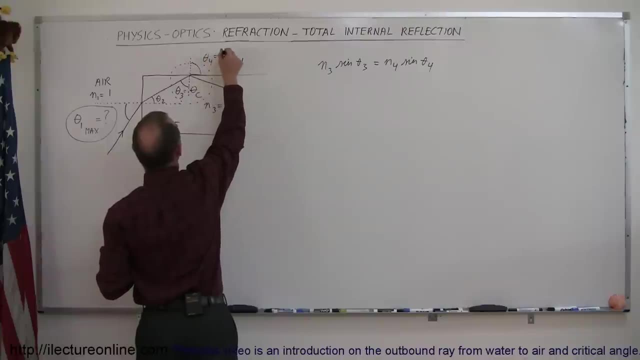 And again, right, we want theta sub 3 to be equal to the critical angle in such a way that if we had a refracted angle, that would be theta sub 4, and we want to make that equal to 90 degrees in order to find the critical angle. 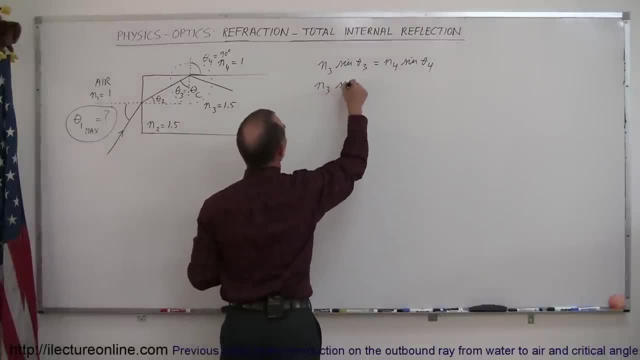 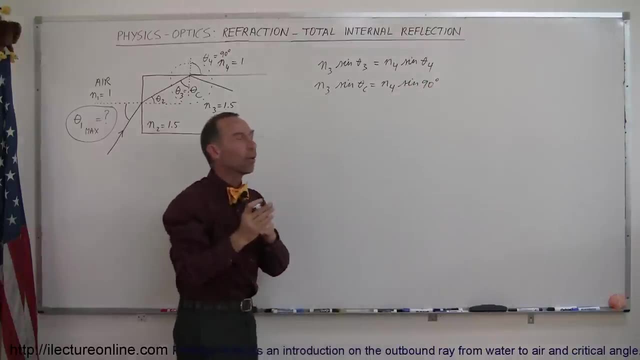 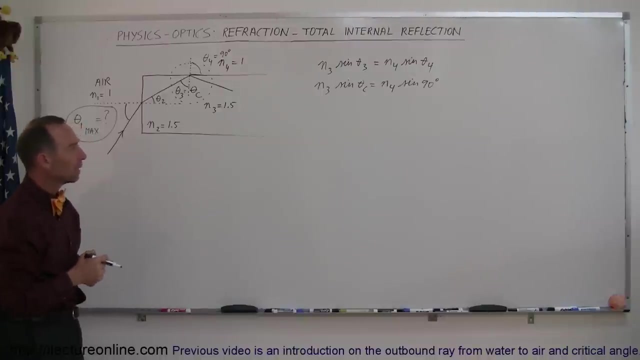 So we say that N3 times the sine of the critical angle is therefore equal to N4 times the sine of 90 degrees. That would be just at the point where the light would then be totally internally reflected. So let's see what theta sub c or theta sub 3 would be equal to, Of course, the sine of 90. 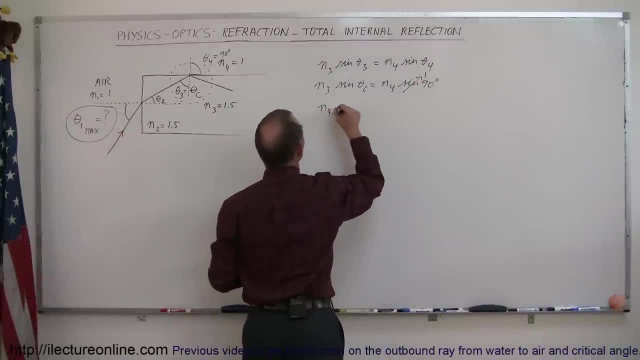 degrees is equal to 1, and so we can say that N3 times the sine of theta sub c is equal to N4. divided on both sides by N3, we get sine of 90 degrees. So that's the sine of the critical angle, is equal to N sub 4 over N sub 3 and finally, the critical angle. 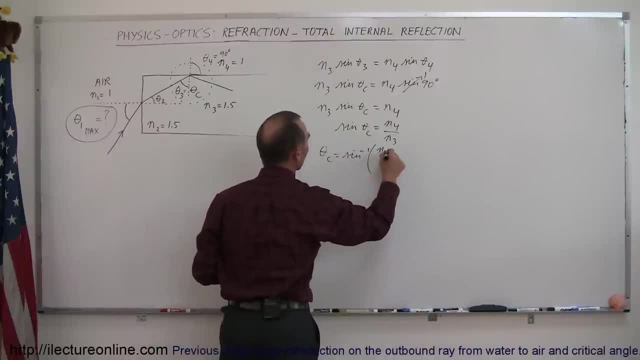 therefore, is equal to the arc sine of N4 over N3.. When we plug in the numbers, that's equal to the arc sine of N4, which is 1, divided by N3, which is 1.5.. So let's see what that angle is for a typical. 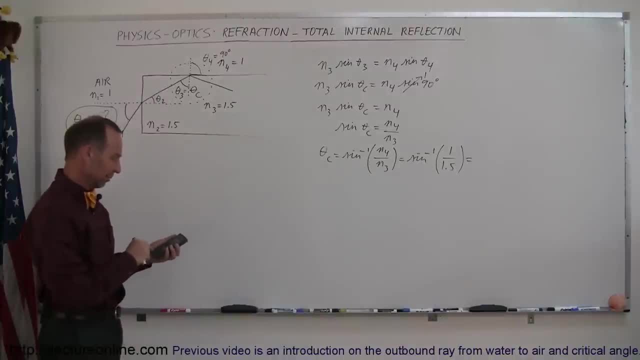 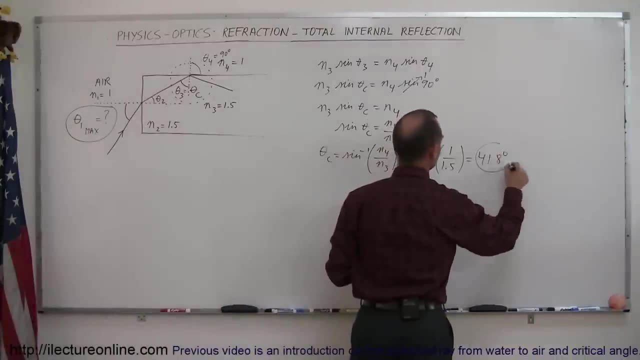 fiber optic cable. So 1 divided by 1.5. take the arc sine of that and we get 41.8 degrees. So that's 41.8 degrees, Which means that the critical angle should be at least 41.8 degrees. that means theta sub 3. 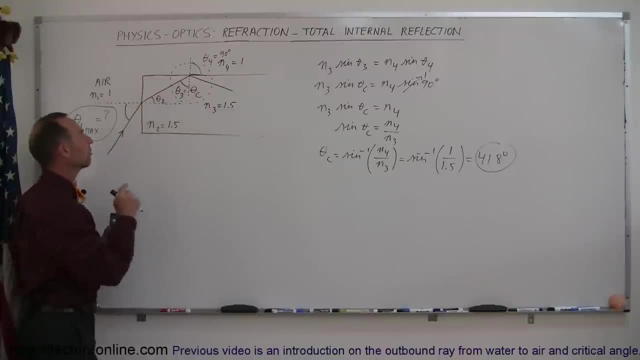 should be at least 41.8 degrees. So if theta sub 3 is 41.8 degrees, what should theta sub 2 then be equal to? So let's take that triangle and draw it right here. There we go. So we have theta sub 3. 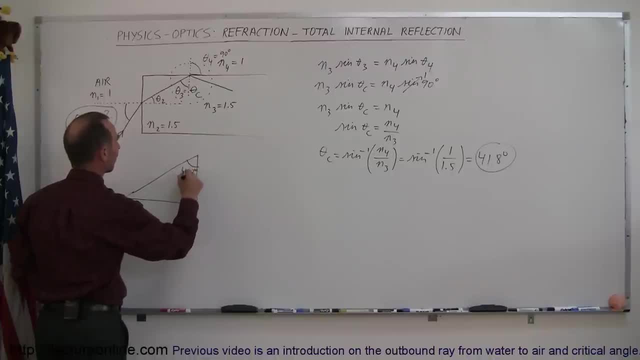 which is 41.8 degrees. We have this angle right here which is theta sub 2, and this is theta sub 2 and we want to know what that is equal to. and of course, you realize in this triangle that this angle plus that angle should add up to 90 degrees, or theta sub 2, therefore, is equal to 90 degrees. 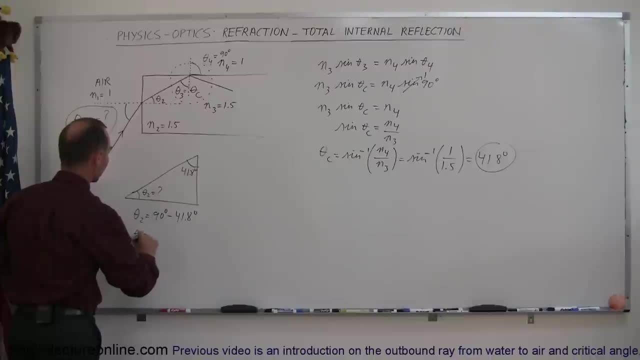 minus 41.8 degrees, which means that theta sub 2 is equal to 48.2 degrees. added those two together you get 90, all right. so theta sub 3 should be greater than or equal to. that means theta sub 2 should be smaller than or equal to 48.2 degrees, which means now we can figure out how much. 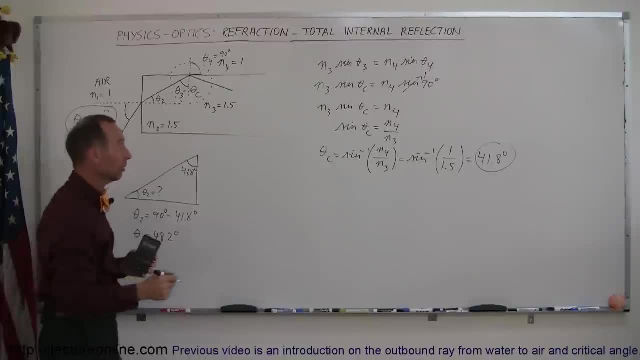 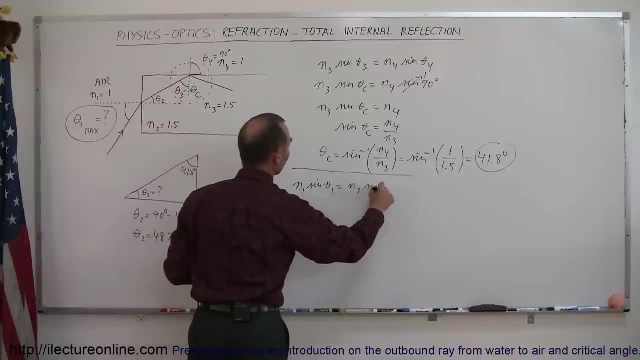 how big theta sub 1 can be. so, again using snell's law, we now write that n1 sine of theta 1 should equal n2 sine of theta sub 2, and let's say we're looking for theta sub 1. that means we're going to 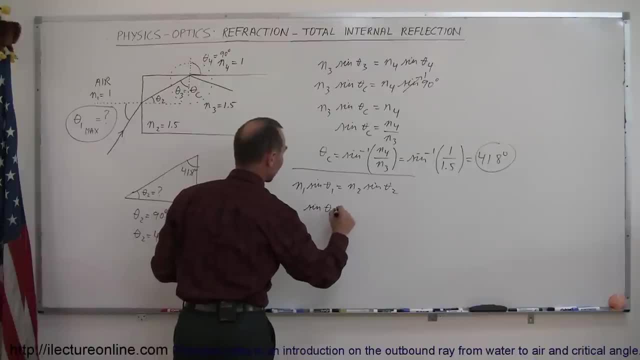 divide both sides by n sub 1. so sine of theta sub 1 equals n2 over n1 times sine of theta sub 1.. sine of theta sub 2: take the arc sine. theta sub 1 is equal to the arc sine of n2 over n1 times the. 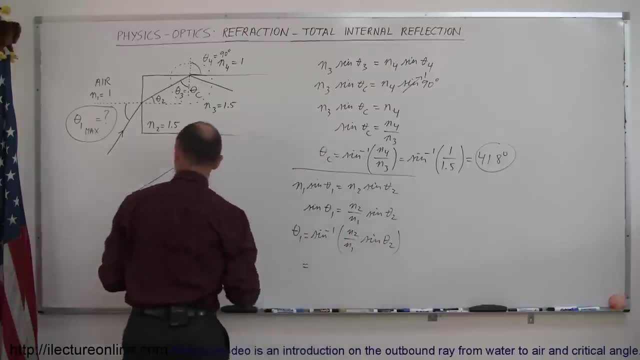 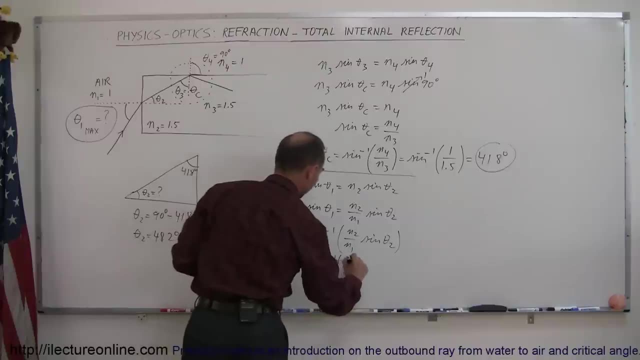 sine of theta sub 2 and plug in the numbers, that is equal to the arc sine of n2, 1.5. n1 was 1 times the sine of theta sub 2, which is 48.2 degrees. and let's calculate. see what that is equal to. 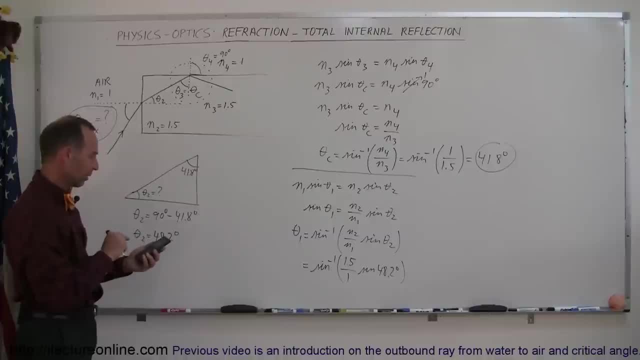 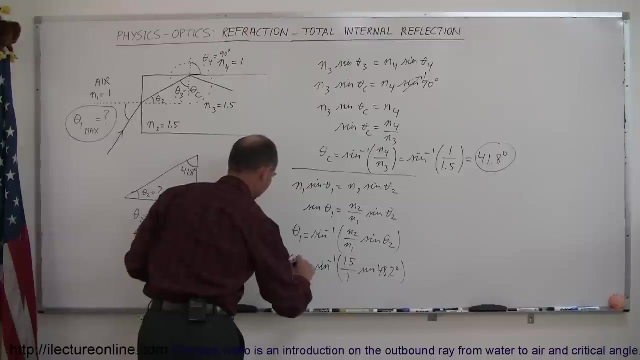 so we made a minus plus 90, so we don't have any runoff errors. then we multiply that. that would take the sine of that. here we go and multiply times 1.5 and wow, we have a problem- actually not a problem. let's see what do we get. so the quantity in here- let me write it down- is equal. 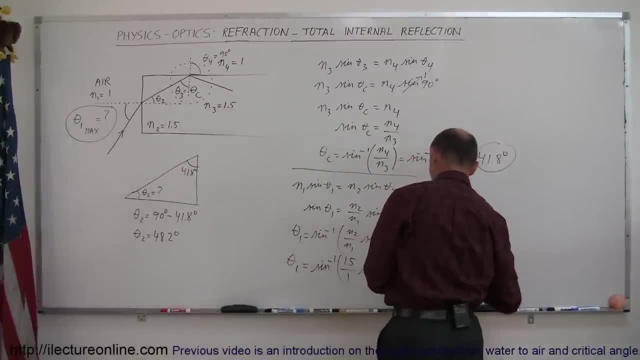 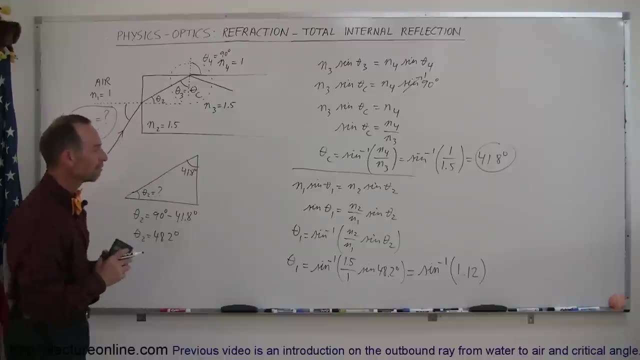 to the arc sine of 1.12. now, of course, we cannot take the arc sine of 1.12. so what does that really mean? well, that means that the angle of incidence has no limit. you can make the angle as large as you want to, because no matter. 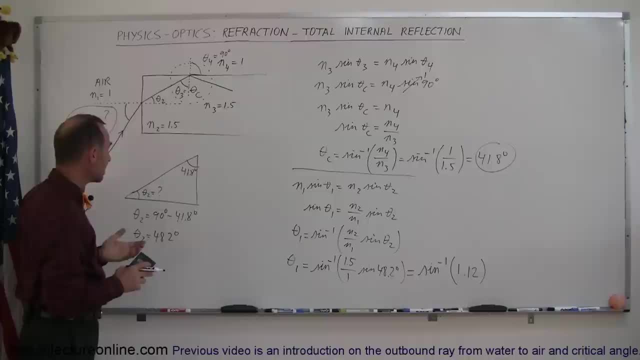 how large you make it, theta sub 2 will never be any smaller than 48.2 degrees, which means that theta sub 3 will never be any larger than 41.8 degrees. all right, so let's just see if we can prove that. Now, let's just see if we can prove that. 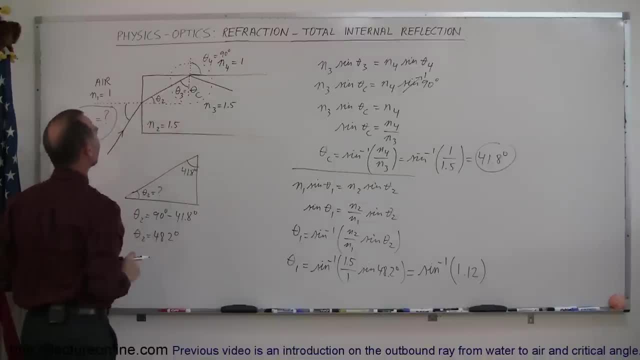 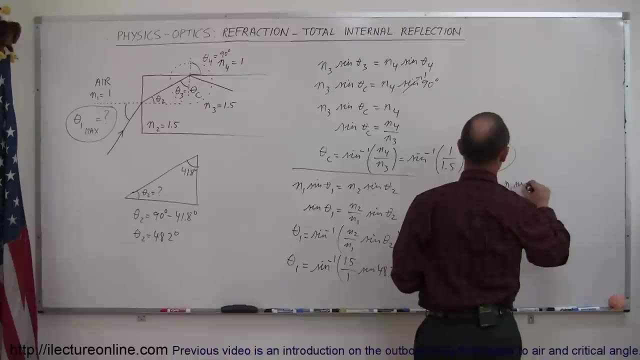 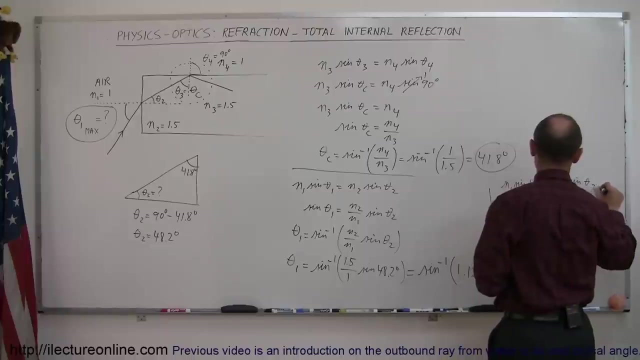 to make theta sub 1 equal to 90 degrees and see what would happen to theta sub 2.. All right, let's do that. So we have the n1 sine of theta 1 is equal to n2 sine of theta 2 and we're going to. 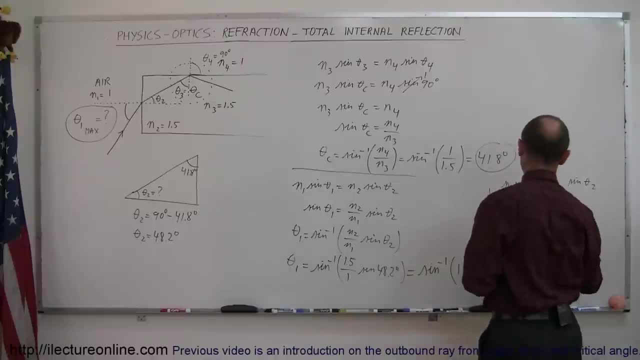 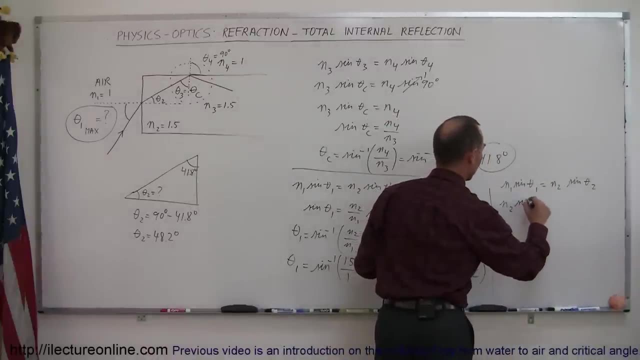 make theta sub 1 equal to 90 degrees and find out what theta sub 2 is equal to. So turning the equation around, let me move out of your way so you can see what I'm doing. So n2 times the sine of theta 2 is equal to n1 sine of theta sub 1.. Defining both sides by n2, we get sine of. 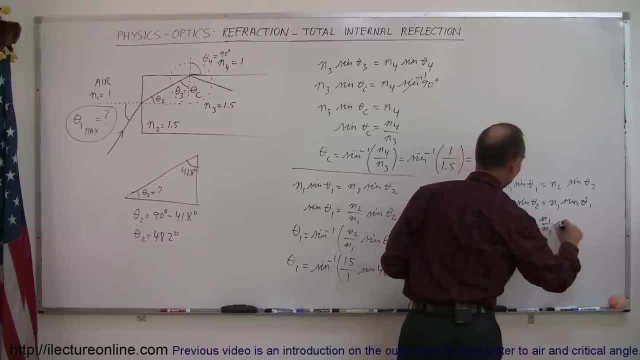 theta sub 2 is equal to n1 over n2 times the sine of theta 1, and so theta sub 2 is equal to going to be equal to the arc sine of n1 over n2 times the sine of theta sub 1.. 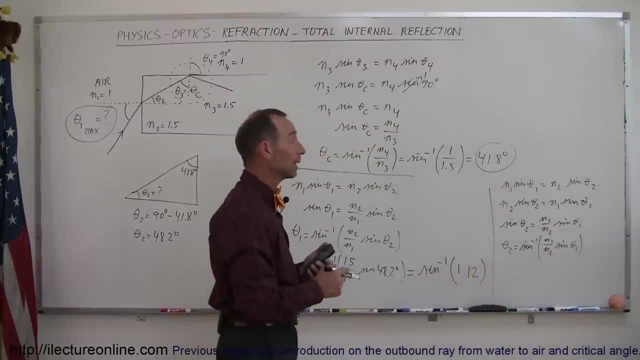 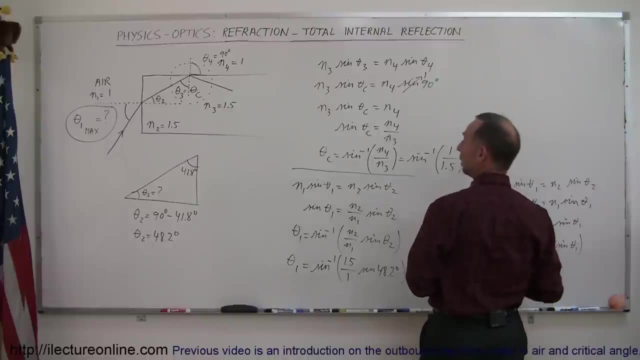 And now we're going to make theta sub 1 as large as we can. so let's make it equal to 90 degrees, and the sine of 90 degrees is equal to 1.. So we're looking for the arc sine of n1, which is 1. 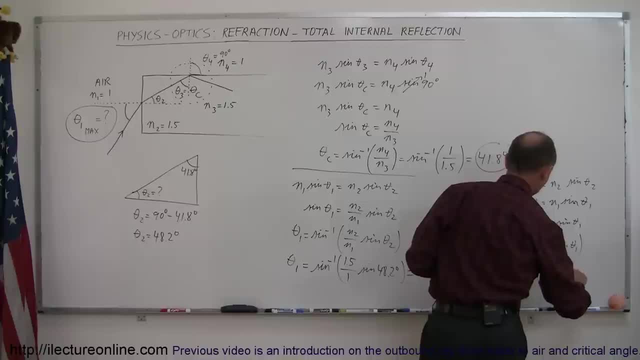 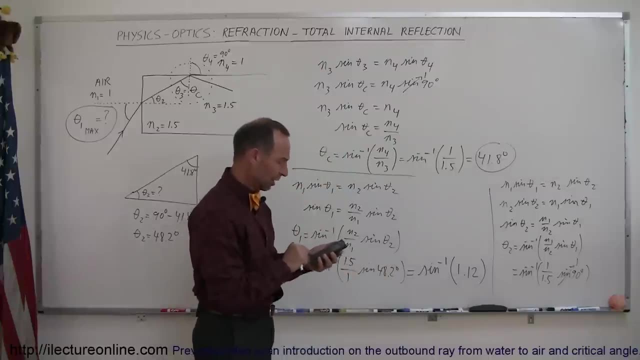 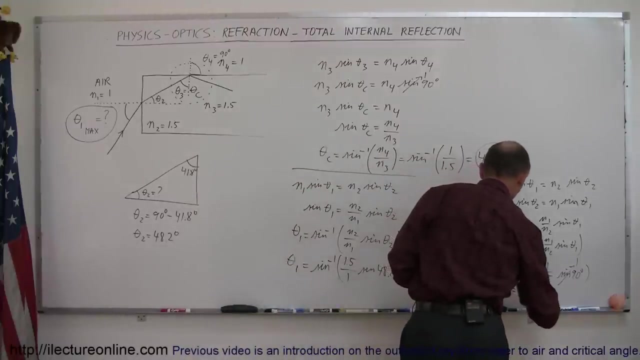 over 1.5 times, of course, the sine of 90 degrees, which is equal to 1, and let's take 1 divided by 1.5 and take the sine arc. sine of that, we get 41.8 degrees. theta sub 2 is equal to 41.8. 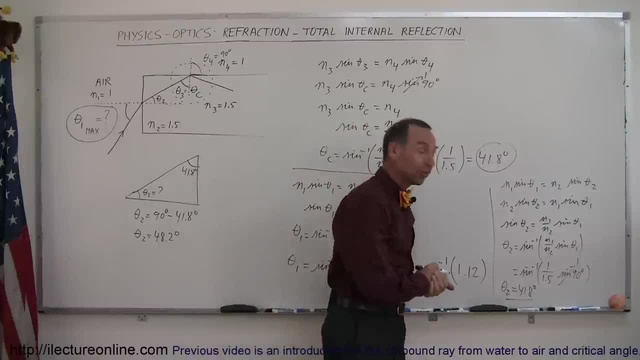 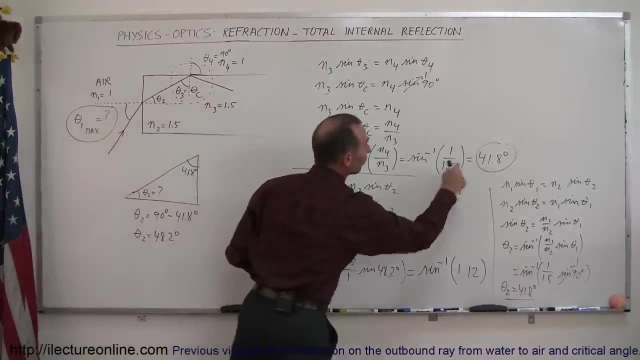 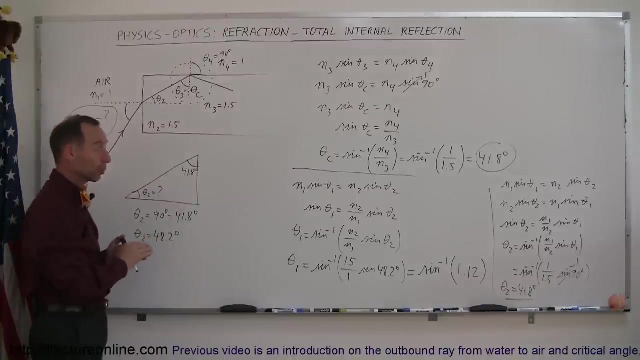 degrees. Okay now, this is a really interesting result, because what we found was that the critical angle needs to be at least 41.8 degrees, which means that theta sub 2 has to be less than or equal to 48.2 degrees, and if we make the angle, theta sub 1 as big as we possibly can, equal to 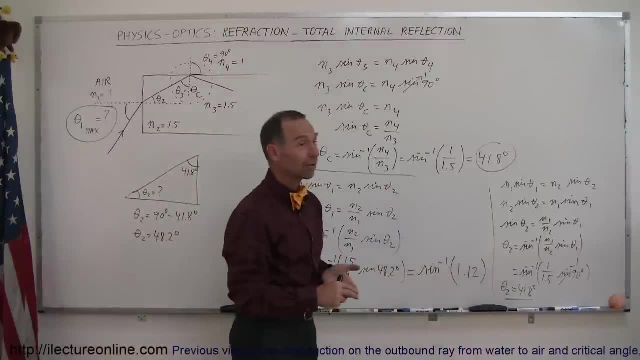 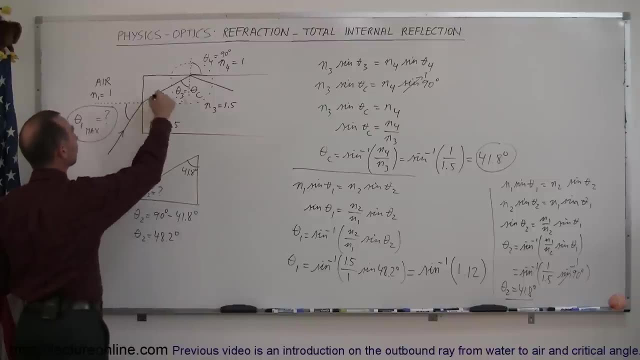 90 degrees. the largest that theta sub 2 can be is 41.8 degrees, which means there is no such thing as a maximum angle. Theta sub 1 can be any angle and as long as you shine light into this fiber optic cable, you will never leave the fiber optic cable and just keep, keep on going. So that's.